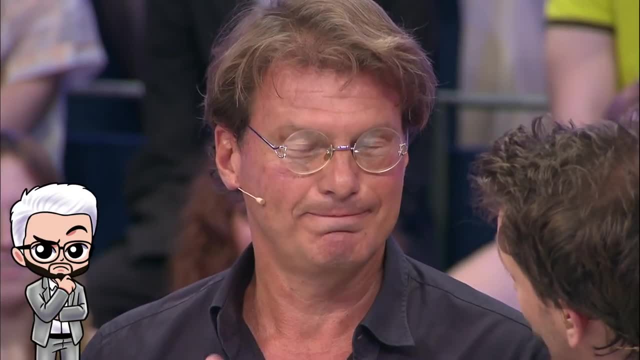 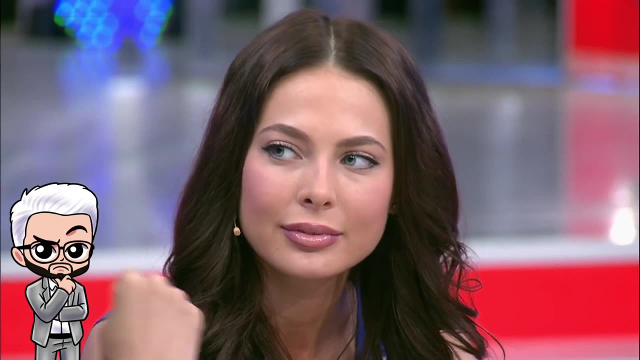 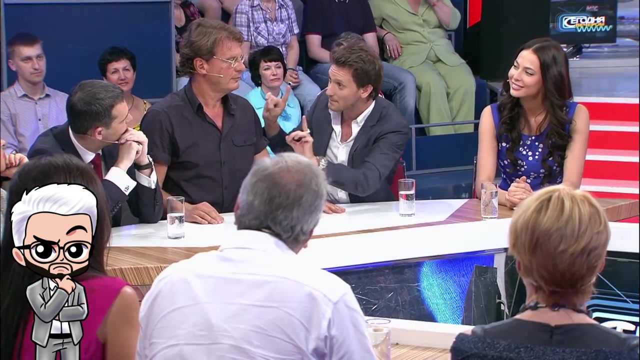 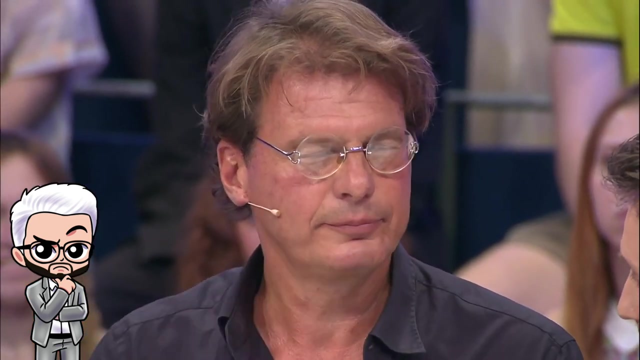 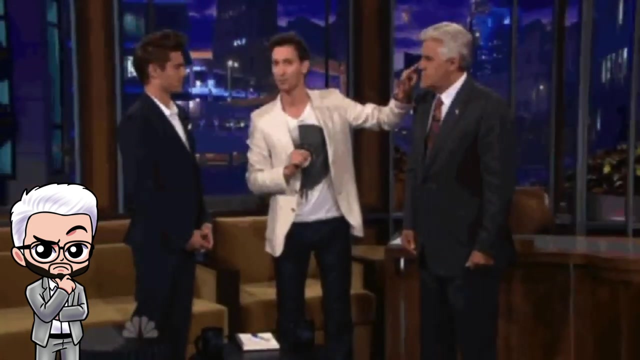 I couldn't get rid of it. Where, Where, Where. I'm going to touch your face in a second. Don't open your eyes, Just tell me if you felt it. You felt a little touch. Can you just point where exactly You felt this On? 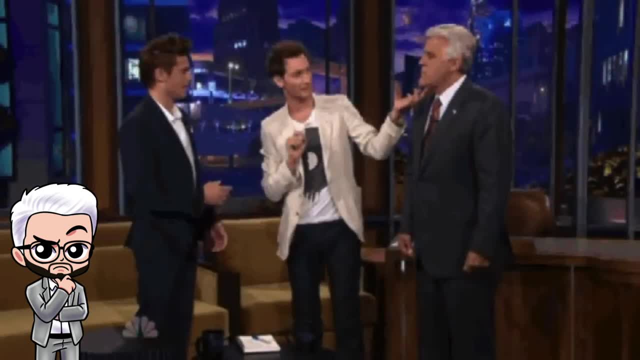 your shoulder. you felt it right. Yes, I feel that You might feel something strange. Tell me if you felt I did. I felt something. You want me to continue or to stop? It's more tickling. I can continue. Should I point, Yeah, Where exactly I felt it right here? 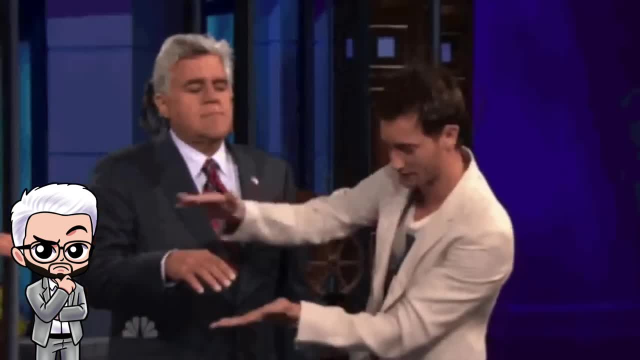 Right over there. Yeah, And just count the number of times in your mind. Don't say it out loud. You can see what I'm doing, I can see what I'm doing. I can see what I'm doing. I can see what I'm doing right now. Tell me if you felt a number of times. Yes, How? 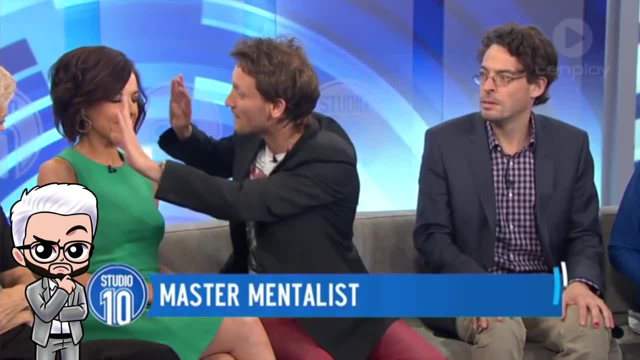 many times. Two: I'm going to touch your face Very, very gently. Don't open your eyes. Don't open your eyes, Just keep your eyes closed. Keep your eyes closed. Keep your eyes closed. You're going to feel a little strange touch, Natasha, Like a little, Did you feel? 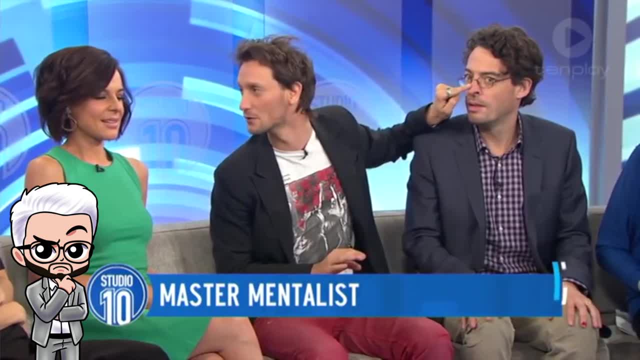 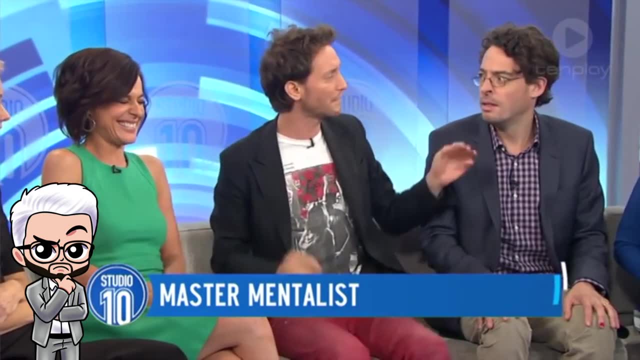 it. Yeah, Yes, Can you show me where did I touch you Here? But don't open your eyes, You might feel Eyes closed, Eyes closed. You might feel a little bit of like a little weird, like a tickling. Where did I tickle? you Just show me where Here. Yeah, That. 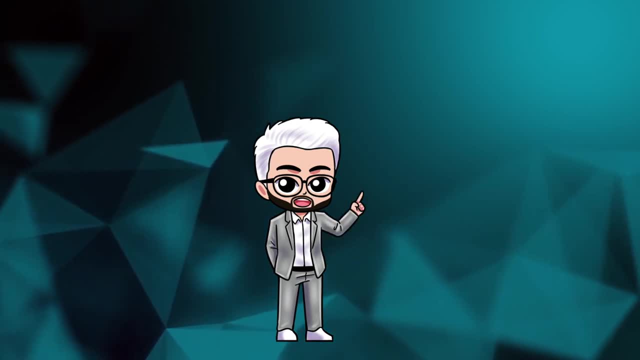 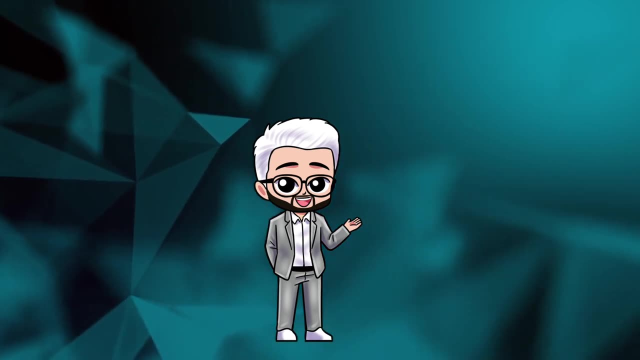 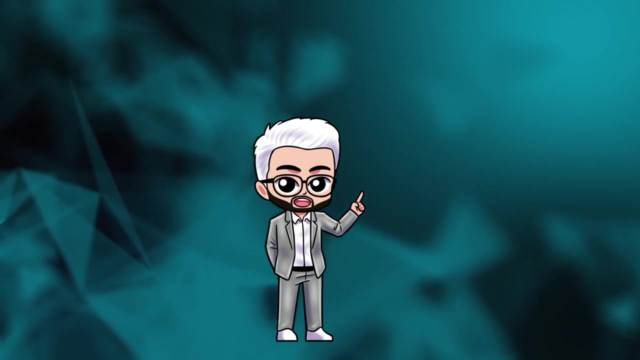 was it. So my job is to show how a regular stage magician that has absolutely no mentalism abilities can do this with simple tricks. Remember, it has to fit the sound and image perfectly, Otherwise I failed. Oh, before we continue, I got to do this bit, Don't forget. 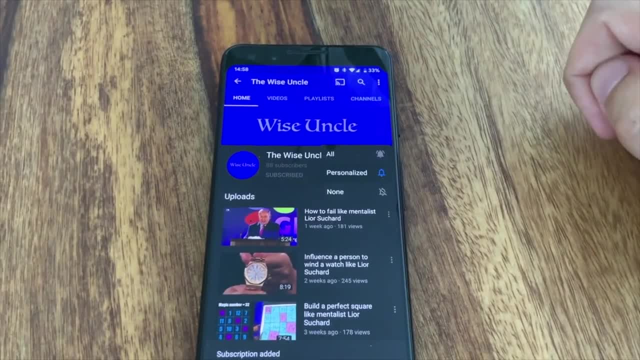 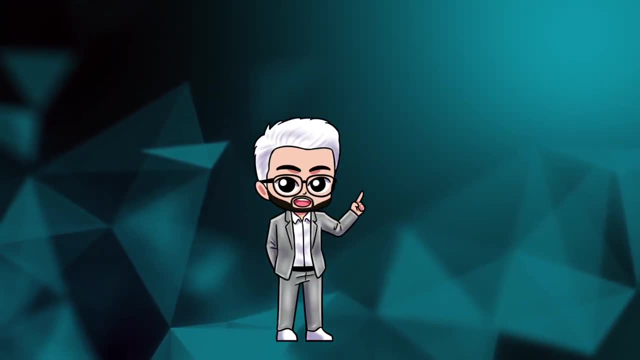 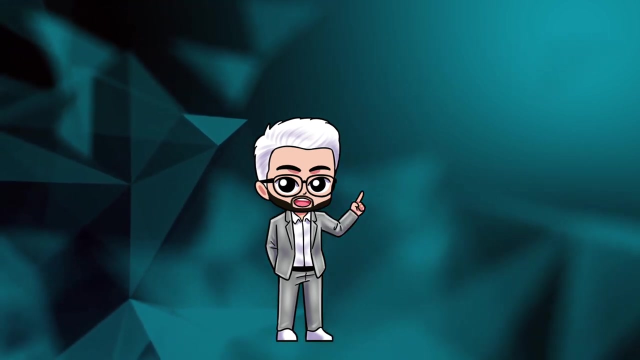 to like, subscribe and click on the bell icon so that you will be notified about new content. Also, if you're willing, you can put links to this channel everywhere you see videos or a discussion about mentalism, Even here on YouTube. I'm not asking you guys to spam. Don't do that. 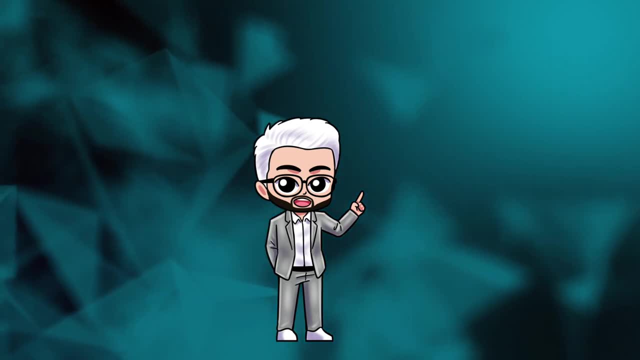 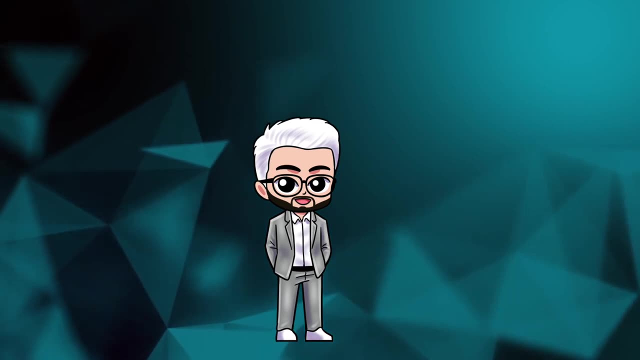 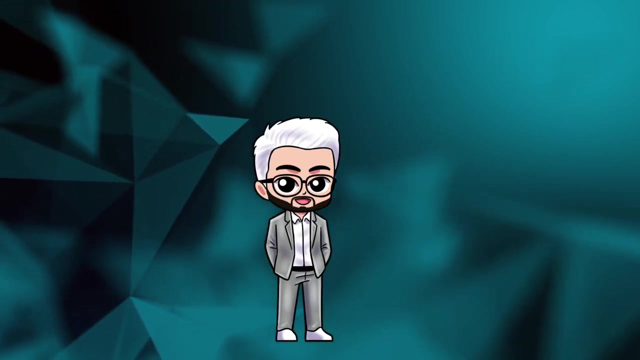 But putting links here and there would be amazing. This is a small channel that would benefit a lot from this kind of support. Now that we got this out of the way, how could this fit be done with tricks? This is the solution. Let's call the person that is being. 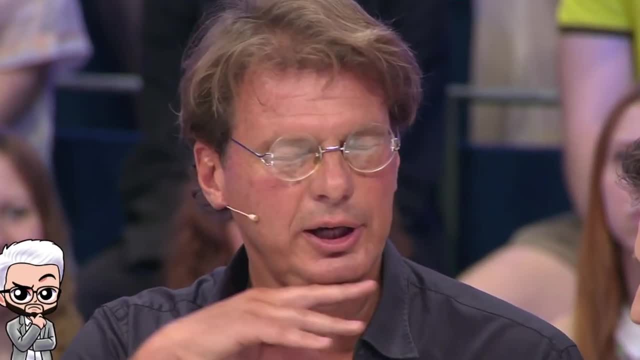 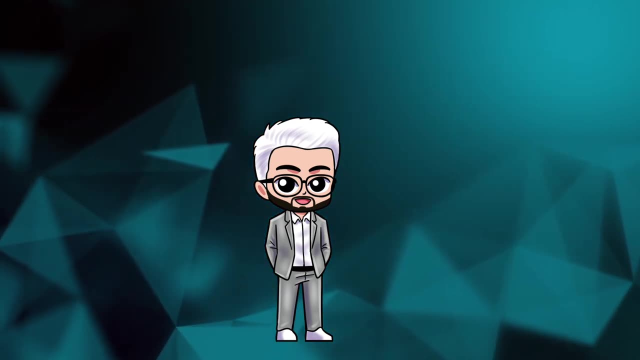 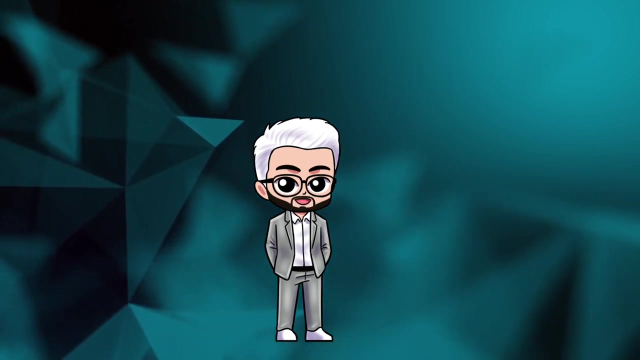 touched Person A and the other person that feels the invisible touch, person B. The magician will first ask person B to close his eyes and then he will touch him with an invisible or almost invisible string gimmick that is between his palms. No one will know that a touch occurred. 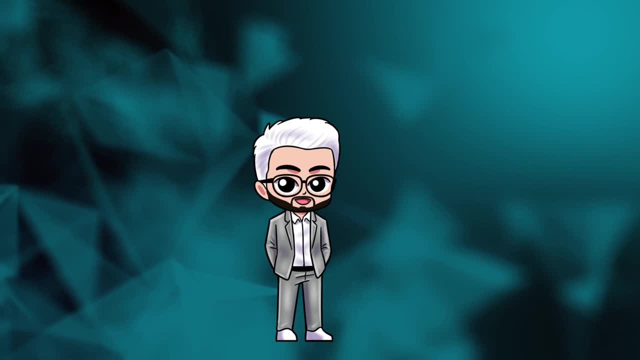 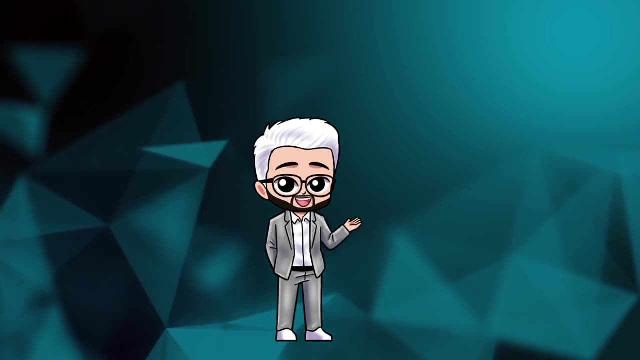 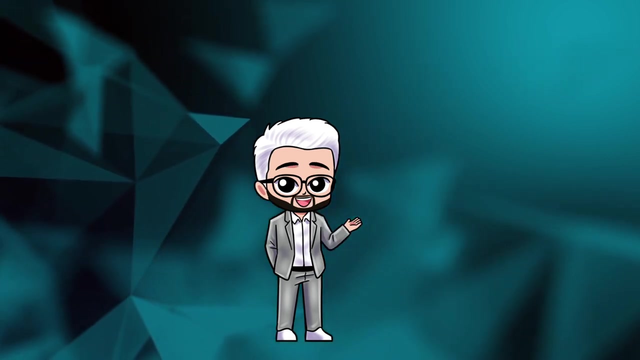 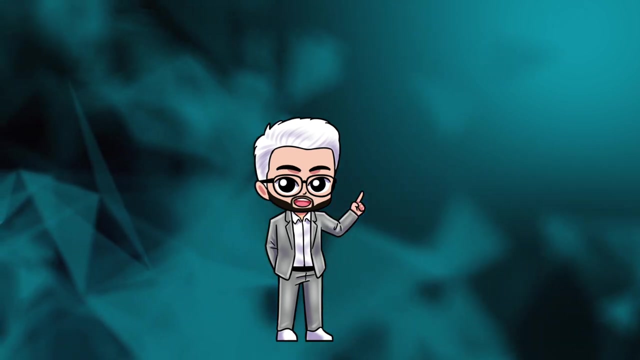 except for the magician and person B. The magician will not ask person B if he felt anything. He will wait with that question until he, the magician, touches person A with his actual hand. After he touches person A, he will ask person B: did you feel a touch? Person B will think that the question is about the touch. 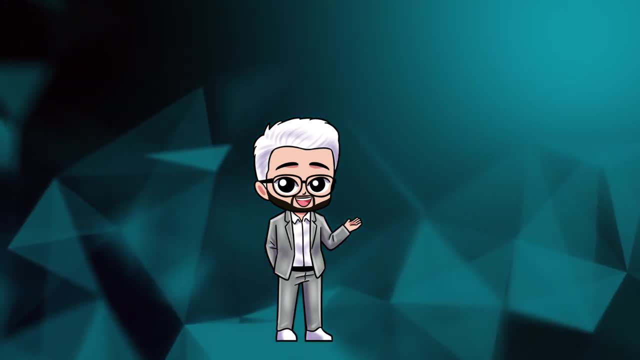 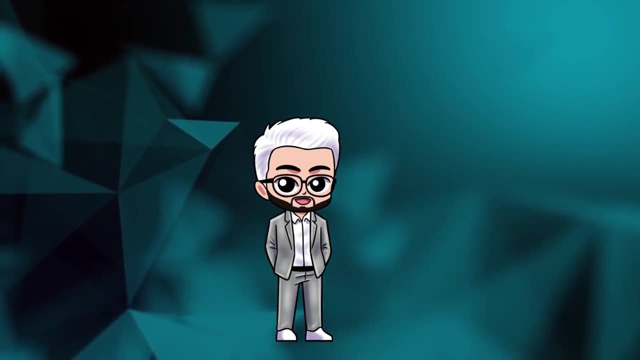 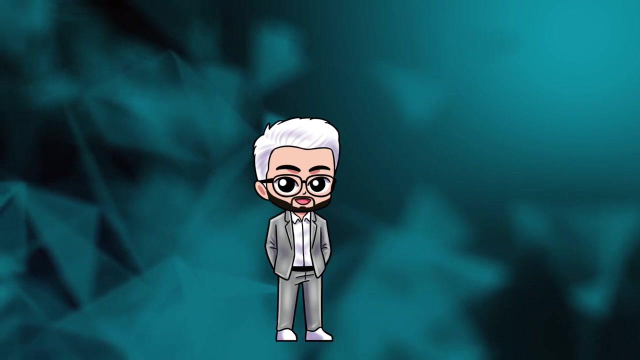 he felt a few seconds ago with the invisible string and he will answer: yes, The audience and person A will think that the report is of a touch he felt right now, where, in fact, he is reporting a touch he felt earlier. Let's watch it again with this new information in mind. 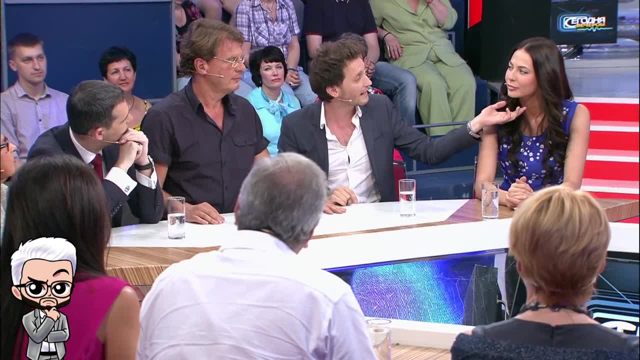 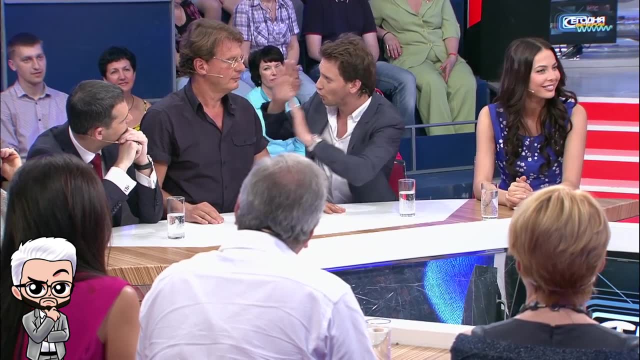 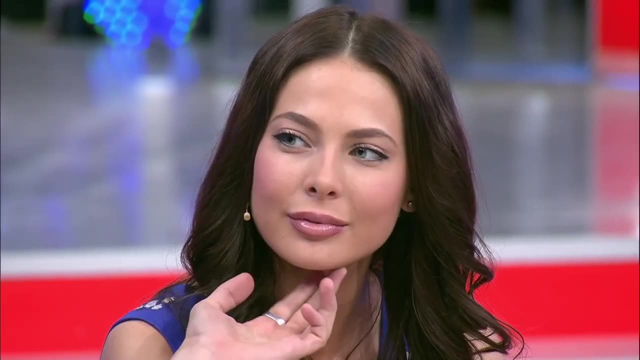 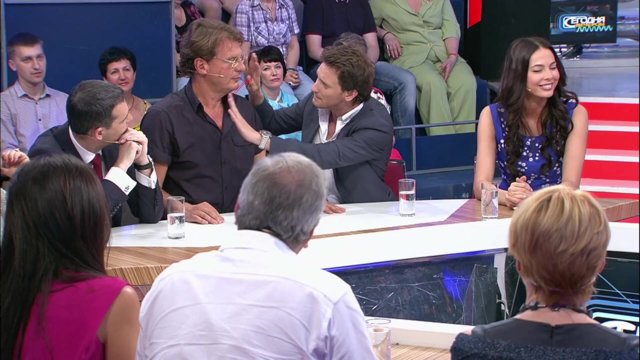 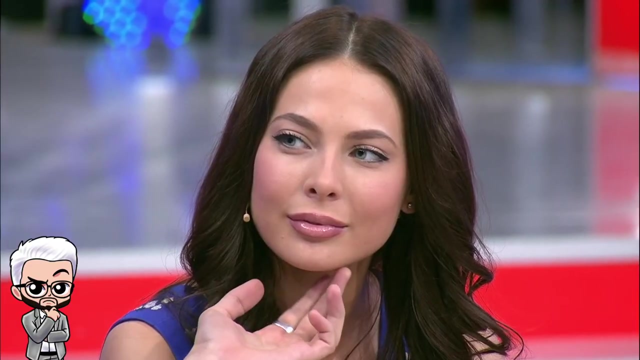 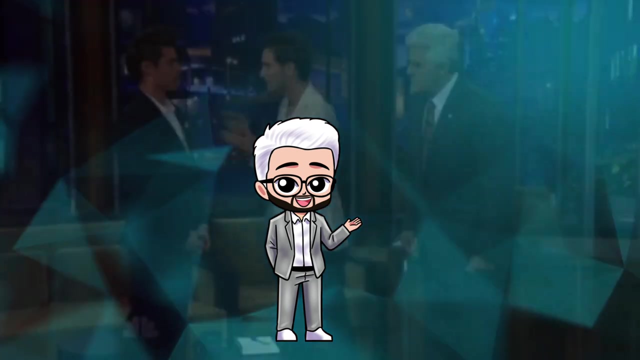 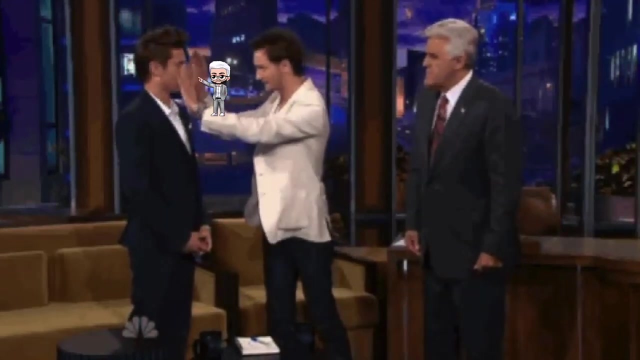 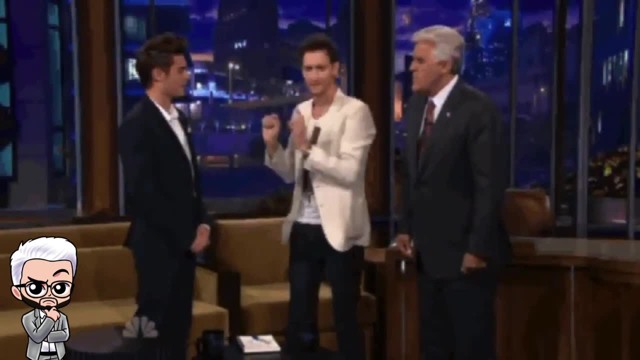 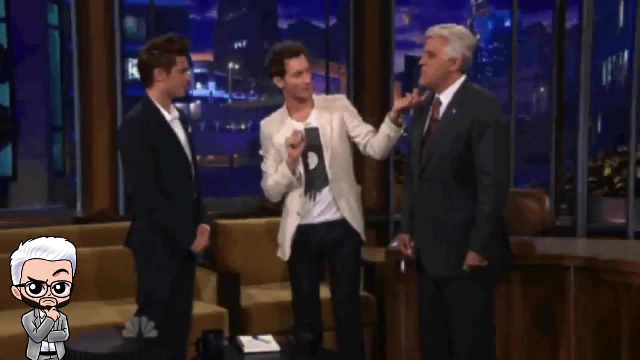 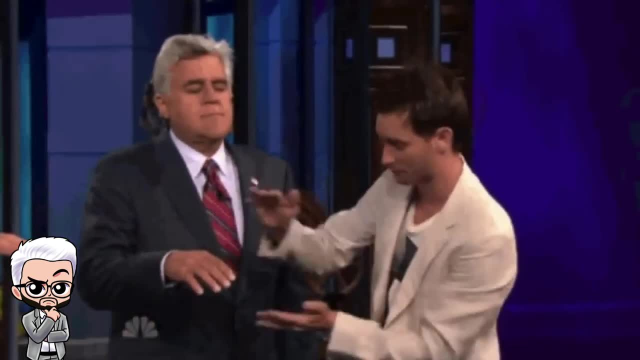 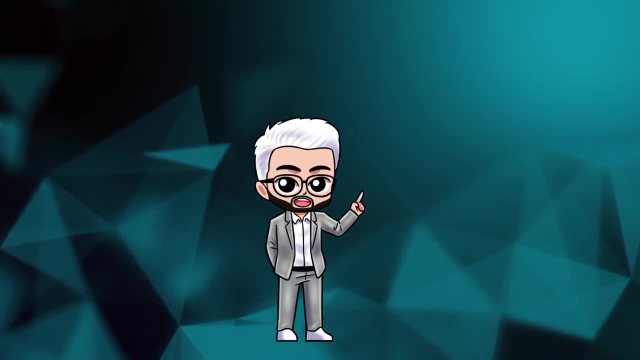 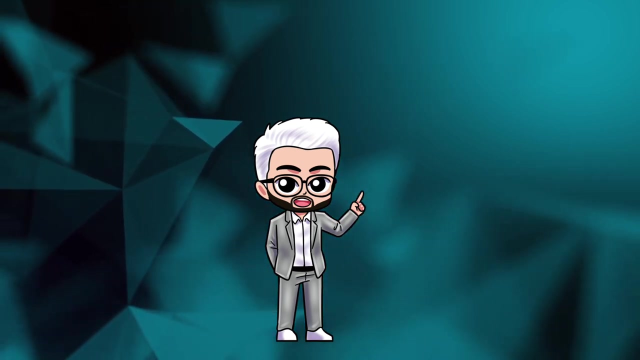 Now in Jay Lennon's show. Now in Jay Lennon's show You probably ask, uncle, if our magician were to use a string, the participant might flinch when he touches him with it. how can you make it fit? Well, check this out. this looked like a flinch to me. if it will happen to our magician. 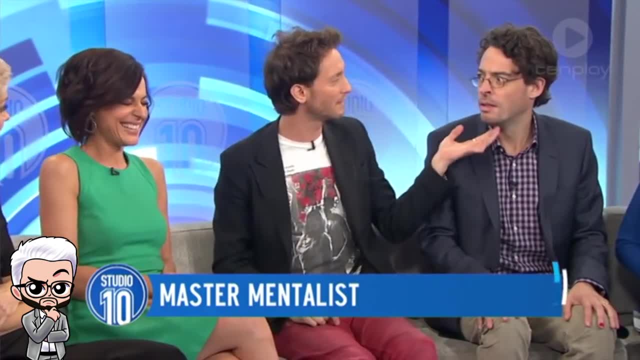 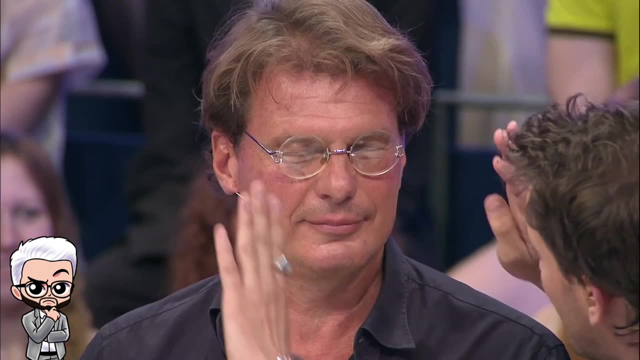 we are clear cause it happened to Sushard- Okay, but wouldn't it happen more than once? It could look weird, right, It might look weird, but it's okay, cause it happened to Sushard more than once also. 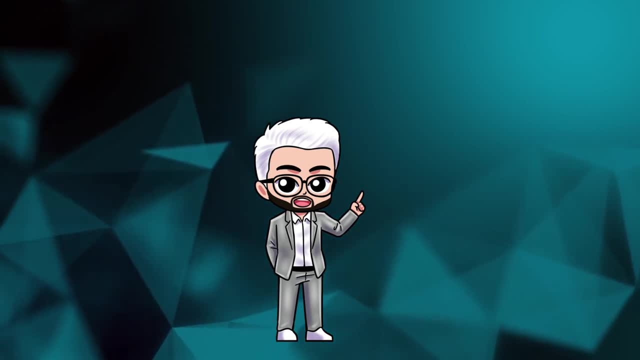 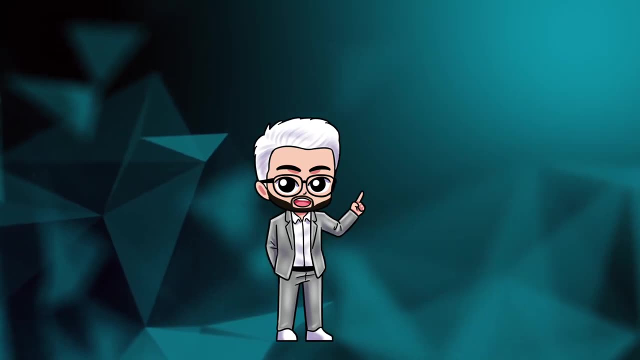 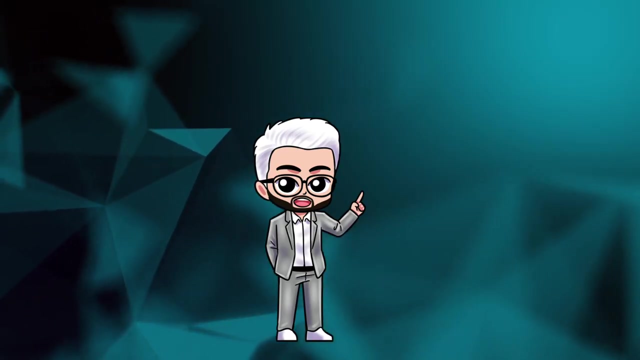 In conclusion, our magician will do the following: he will use invisible string gimmick to touch a participant without the audience knowing. He will then continue to touch the other participant visibly with his hand and only then he will ask the first participant if he felt something. 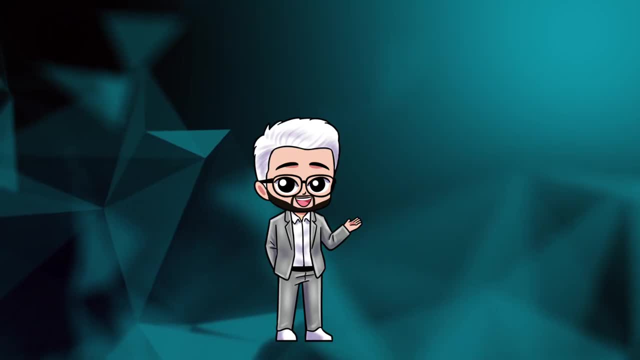 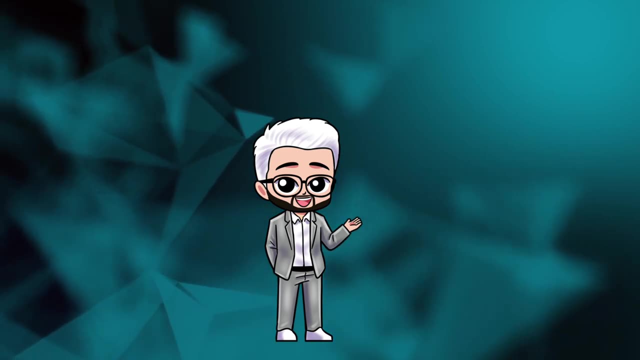 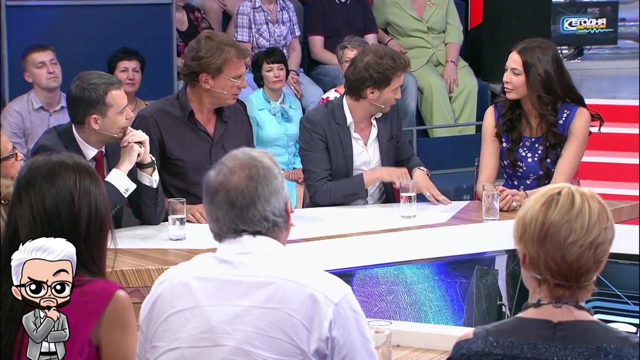 The first participant will answer yes, and that's it. The illusion is complete, without any mental abilities, and it would not look any different than what Sushard did: Mission, Mission, Mission, Accomplished. If you feel something strange around midnight tonight, 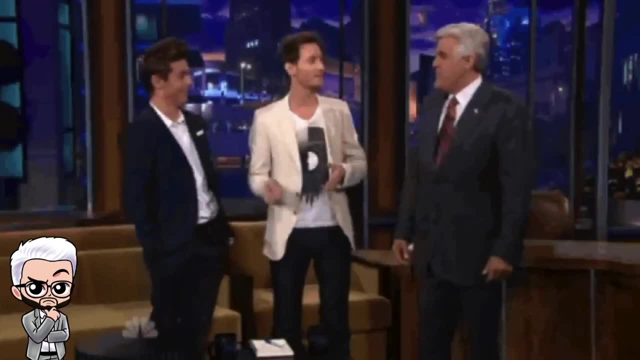 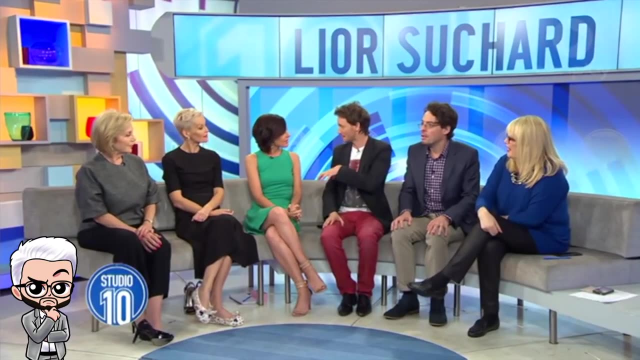 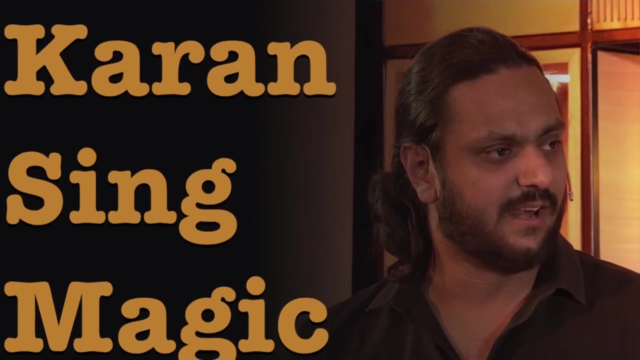 not today. so this means that every place you touch yourself for the next week, you know what this means. If you feel something strange around midnight tonight, it's not me, it's probably him. Next video we will review Karan Singh magic. 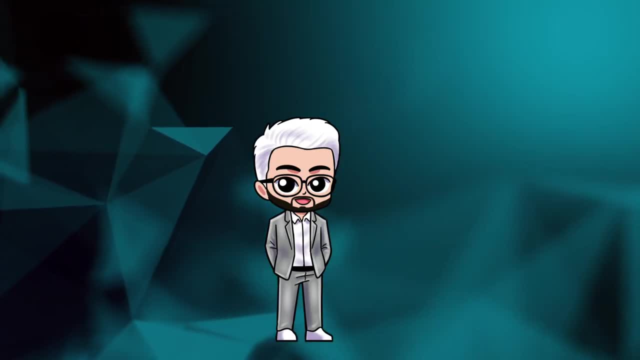 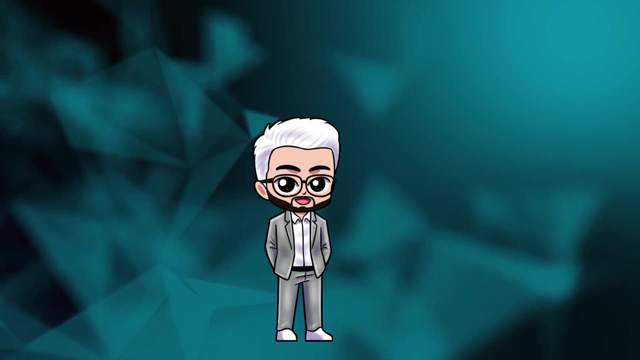 If there is a specific video you want me to do, you can put it in the comments below. So I was your wise uncle. if you liked this video, you should watch my other Leo Sushard videos. we accumulated quite a lot.